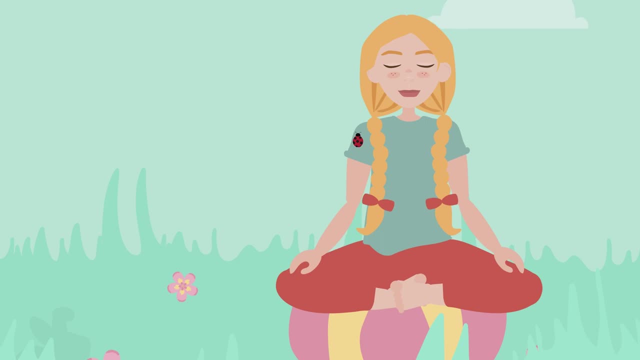 can be any color you want it to be. this is your happy place. everything is exactly how you want it to be. your ladybug friend is here to help you relax. can you feel your little ladybug friend on your shoulder? feel their tiny legs gently tickling you? let's play a game with your ladybug friend. 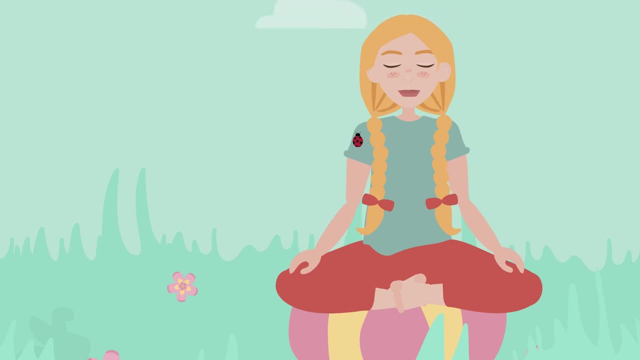 every time your ladybug friend lands on a different part of your body, go ahead and relax that body part. go ahead and relax the shoulder you're ladybug friend is resting on. now your ladybug friend flies into the air and lands on your hand. relax your hand as it gently crawls to your fingertips. 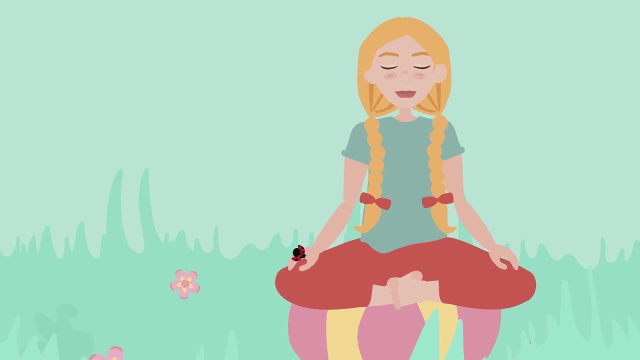 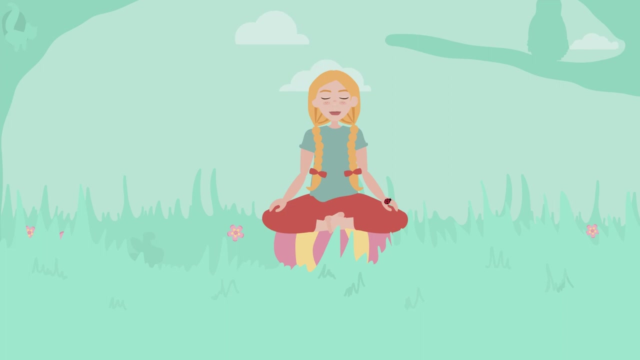 wiggle your fingertips and let the ladybug friend fly back into the air. Now your ladybug friend flies and lands on your other shoulder. Relax that shoulder. Now your ladybug friend flies into the air and lands on your other hand. Relax your hand as it gently crawls to your fingertips. 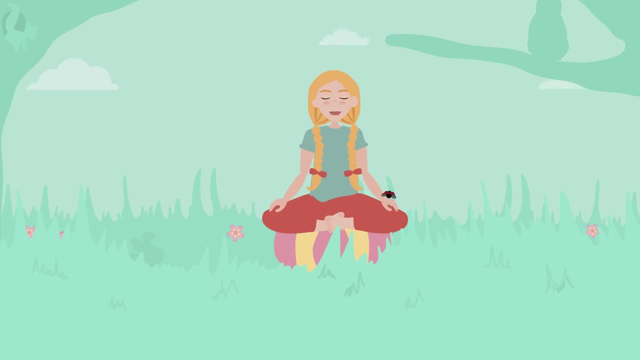 Gently wiggle your fingertips and let the ladybug friend fly back into the air again. Now your ladybug friend flies and lands on your knee. Go ahead and relax your knee as it slowly crawls to your toes. Give your toes a little wiggle. 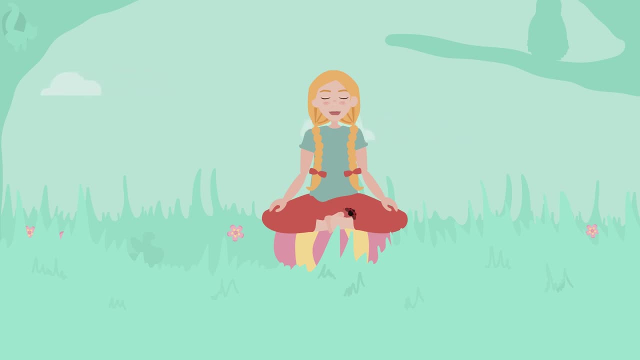 And relax your foot as your ladybug friend flies to your other knee. Relax your knee while your ladybug friend slowly crawls to your toes. Now give those toes a wiggle And relax your foot as your ladybug friend flies slowly to your tummy.